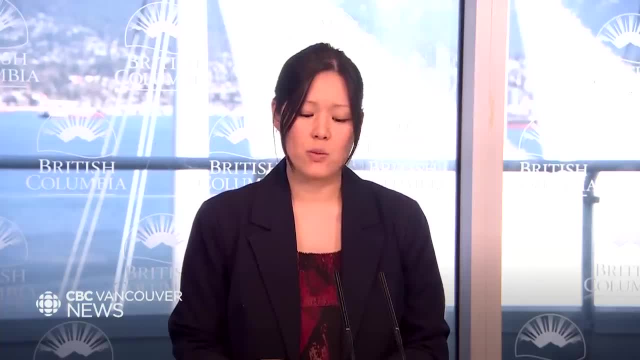 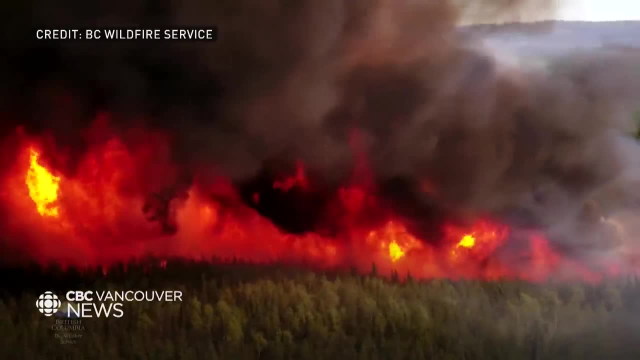 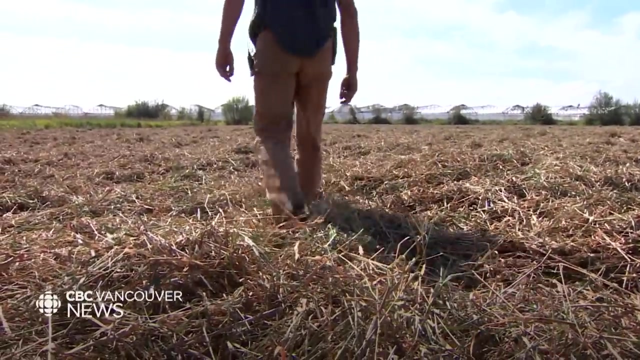 we are taking action earlier than ever, and preparations for this year's wildfire and drought seasons are already underway. There are obviously opportunities for much more waiting to come, but the sustainability of land that can be reimbursed in place with thedi pots has consistently since been well underway. 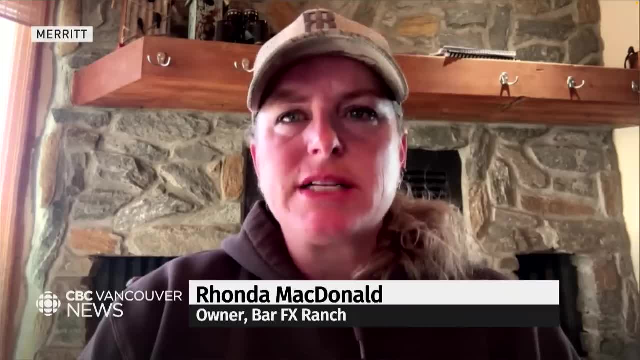 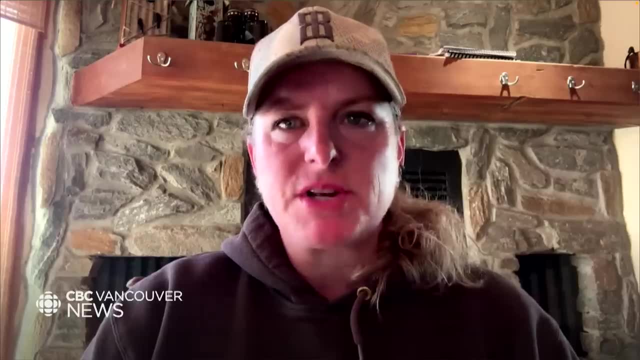 Anticipating wildfire: BC announced plans to train volunteers and help people who are forced to flee their homes. Anticipating drought: cash is promised for the agriculture sector, But what ranchers really want is rain. Aanticipating wildfire: BC announced plans to train volunteers and help people who are forced to flee their homes. Anticipating drought: cash is promised for the agriculture sector, But what ranchers really want is rain. Those insurance programs designed to cover are bare costs. only, You can't make a living at it, You know. we just want to do what our jobs are, and that's to grow food for people who aren't making a living. Costa, there's more sushi. 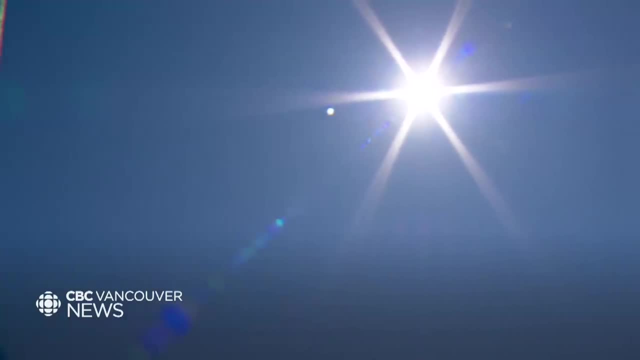 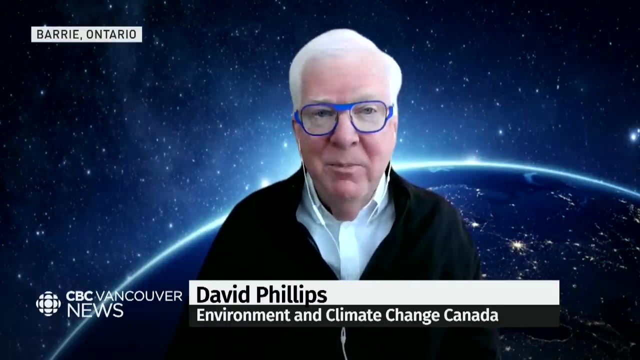 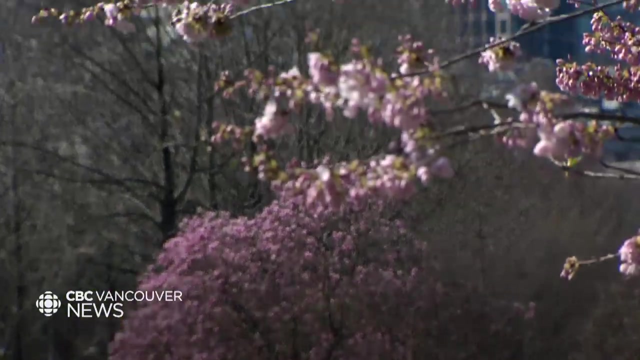 people and animals. Environment. Canada says this heat could stick around. Our models are out and we're saying that. no cold areas. we're seeing every part of Canada. it looks like it's going to be warmer than normal. That means warm Sun, early blossoms, spring joy tinged with worry. Lindsay Duncombe, CBC News. 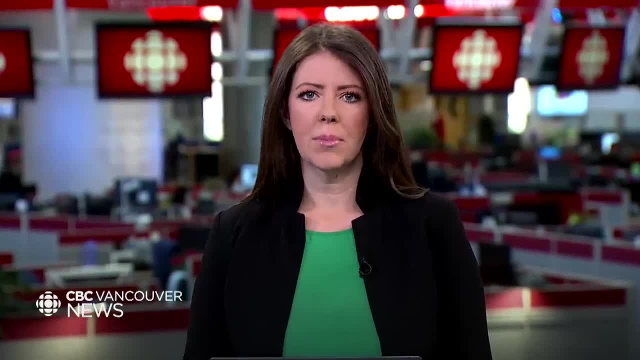 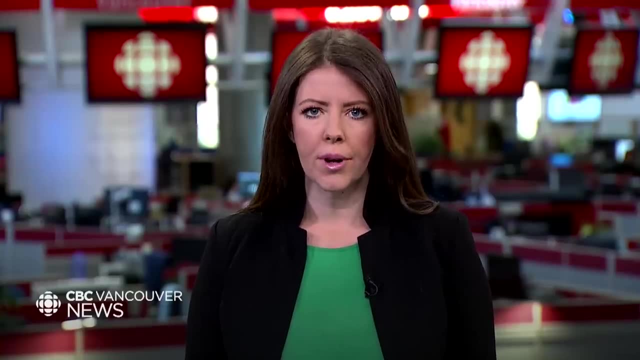 Vancouver. As Lindsay mentioned, the summer-like conditions have the province mobilizing to prepare for this year's wildfire season. New strategies and updated protocols are being rolled out and it appears more help may be on deck than before. The BC wildfire service has received double the number of. 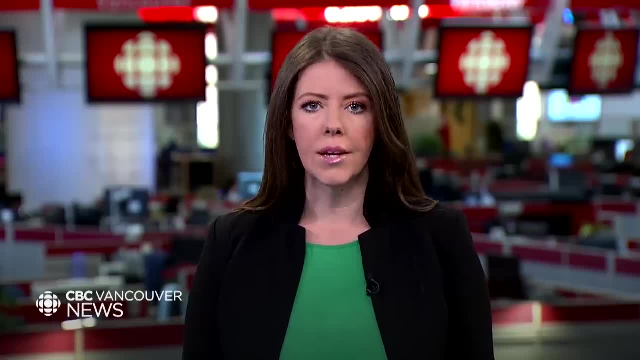 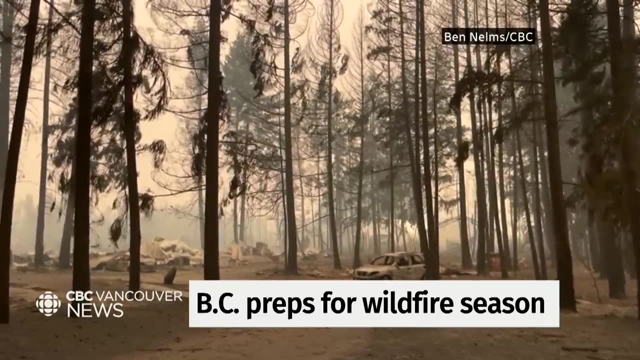 applications. this year, compared to last, Mira Baines continues our coverage. The province is preparing for this year's wildfire season, after last year's became the worst, most destructive in BC's history. In fact, we are taking action earlier than ever and preparations are underway. 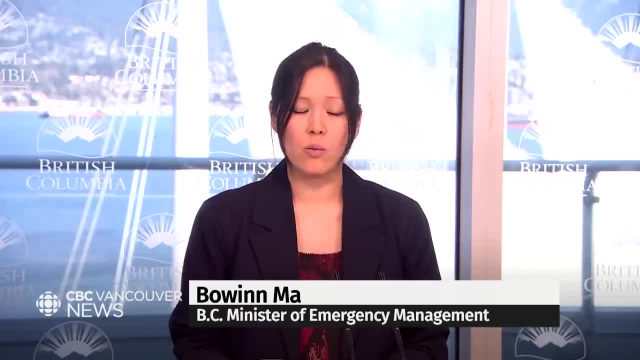 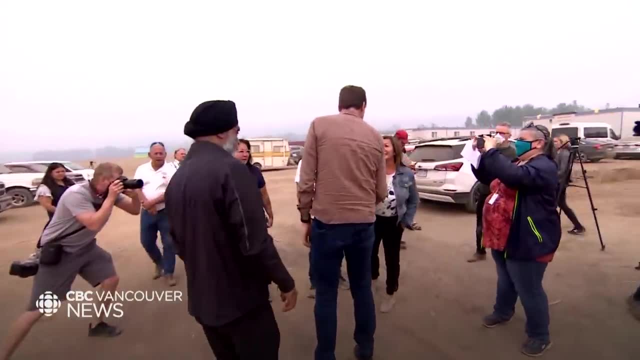 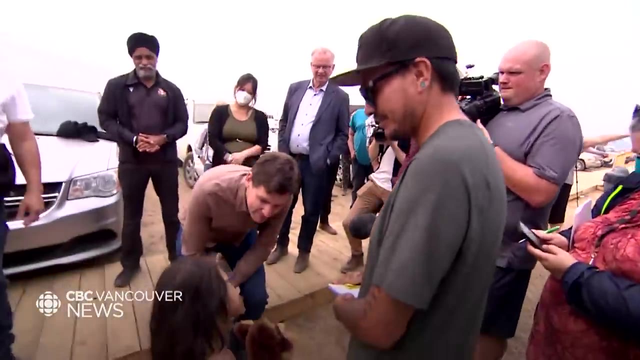 For this year's wildfire and drought seasons are already well underway. Tens of thousands of people were forced to evacuate from their communities and hundreds lost their homes. The provincial government was criticized for lack of timely emergency response and supports for people who had to flee, Now hoping to 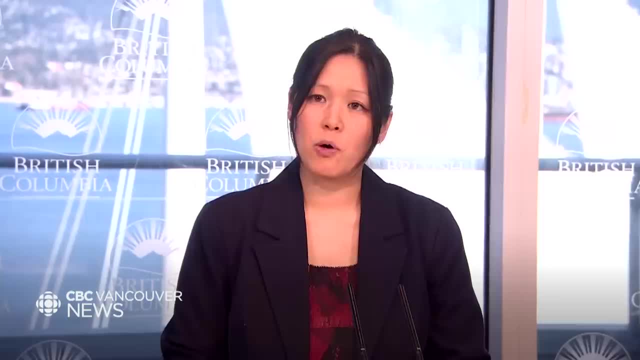 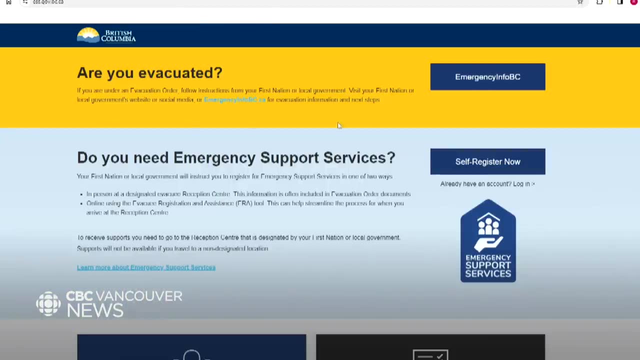 change that. That's why an expanded team of emergency support specialists within my ministry is wet ready to be deployed to communities who need that extra support. It's encouraging people who feel they could be at risk for evacuation to create an online profile on the emergency services website so they can